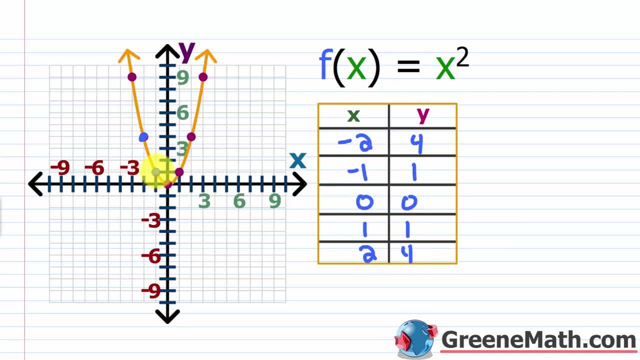 my negative 2, 4 here. I have my negative 1, 1 here, My 0, 0 here, My 1, 1 here And my 2, 4 here. I also have my negative 1, 1 here And my 2, 4 here And my 2, 4 here And my 2, 4 here And my. 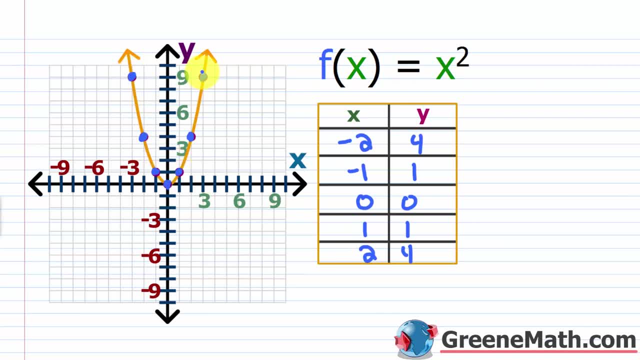 negative: 3, 9 right there And my 3, 9 there. So I can't fit all that here because I'm out of space And we only need a few of these values to kind of compare in our next section. anyway, 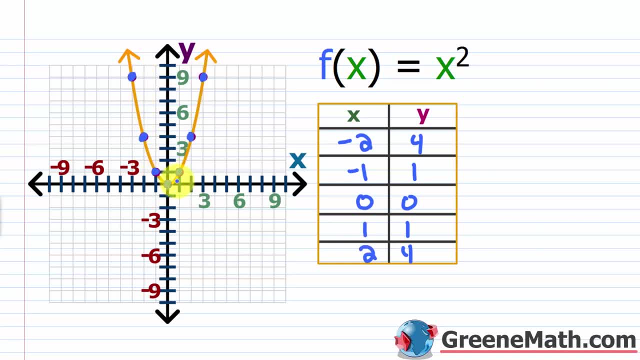 But I just want you to get the idea here. These are the kind of basic points that you should associate with y equals x squared or f of x equals x squared. So every time you want to graph this guy, you know these points by heart And you can kind of sketch this graph very quickly Now. 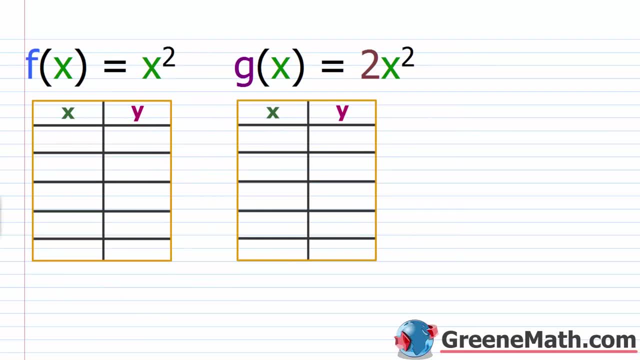 knowing that we've committed f of x equals x squared kind of to memory. we know the points associated with it. We know the shape. Suppose we had a new function where we take this original function and we multiply the right side by 2. So in other words, we have f of x equals x squared. 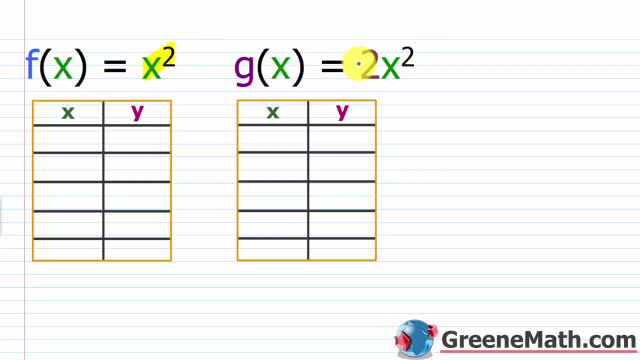 So focus on this x squared part. Now we have g of x equals 2 times this x squared. So essentially I can write g of x by saying it's 2, this number right here times f of x. What's f of x? It's x. 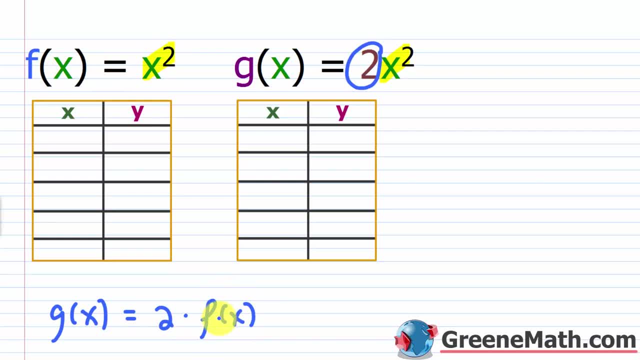 squared, So times f of x. You'll see this notation in your textbook, And what's going to happen is this is going to give us a vertical stretch, And I'll explain why in a minute. But essentially, for the same x value, the y value is now going to be twice as. 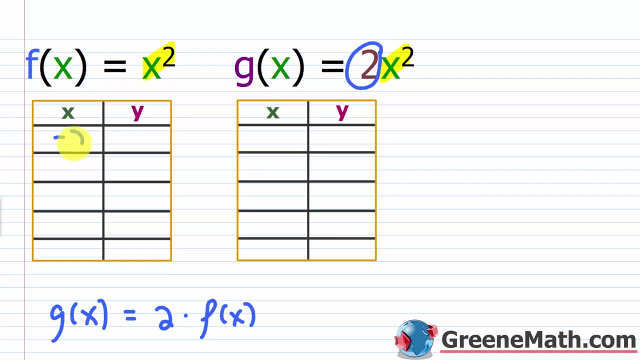 large. So we filled out this table of values. before We said negative, 2, 4.. We said negative 1,, 1,, 0,, 0,, 1,, 1, and 2, 4.. So if I keep the same x value, so negative 2,, negative 1,, 0,, 1, and 2,. 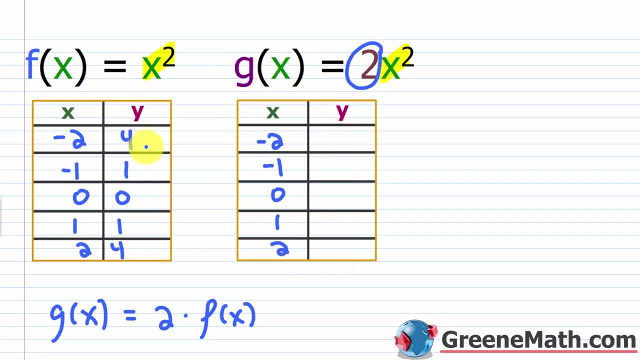 the y values here now for g of x will be twice as large as the y values for f of x, again given the same x value. So instead of a y value of 4 when x is negative 2,, now it's going to be 8.. And again, think about why that's the case. I plug something. 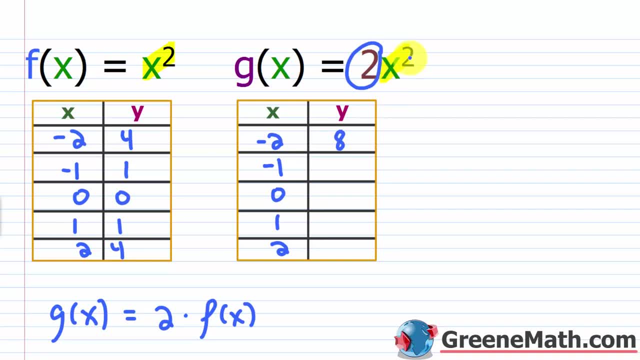 in for x. I square it Now. instead of getting my output, I still got to multiply it by 2, OK, So the original output is multiplied by 2. And now I have my output. OK, So that's why I can. 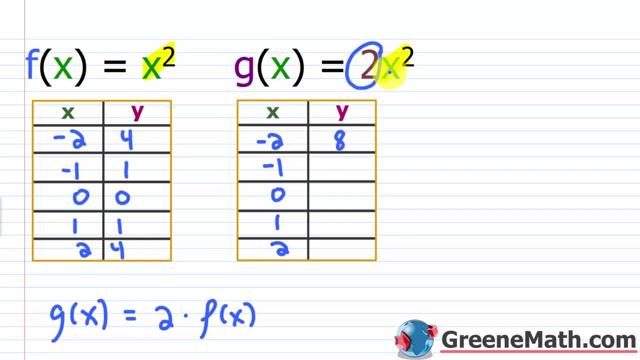 take this y value of 4, multiply it by 2 to get 8.. Negative 2 squared is 4.. Then times 2 would give me 8.. So this guy 1, would now be negative 2.. And now I have my output, which is negative 2,. 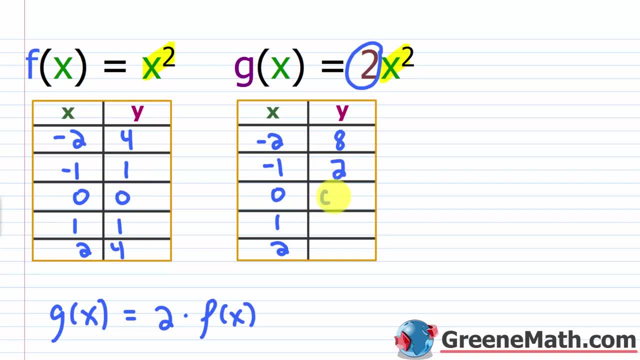 times 2.. So that's 2.. 0 times 2 is still 0. Then 1 times 2 is going to give me 2. And of course, 4 times 2 is going to give me 8.. So again, for the same x value, y is going to be twice as large. 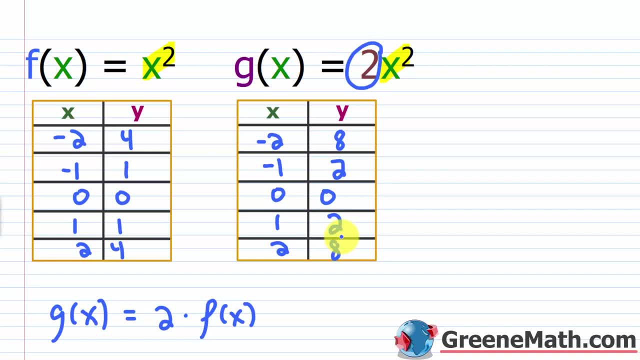 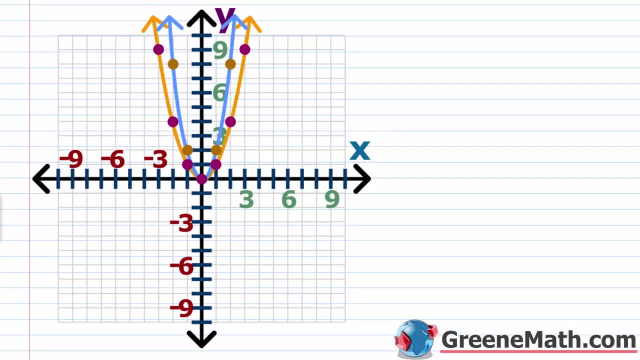 So this is going to create a graph that is vertically stretched. When compared to f of x equals x squared, you're going to see that it's skinnier or narrower, So let's take a look at this visually. So the guy in orange- this is my original- f of x is equal to x squared, So this: 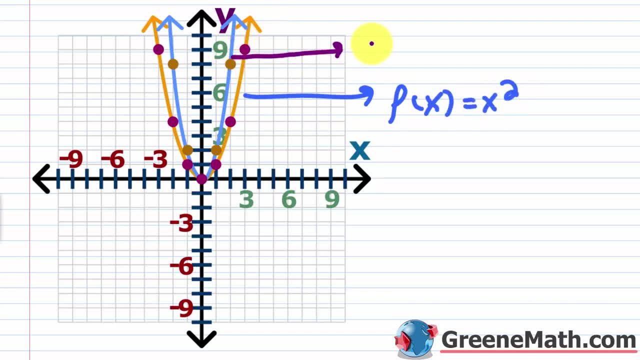 guy in light blue. this is my. g of x is equal to 2 times x squared, Or really we could say g of x is 2 times f of x. OK, So this multiplication of 2 times this function f of x is what's creating. 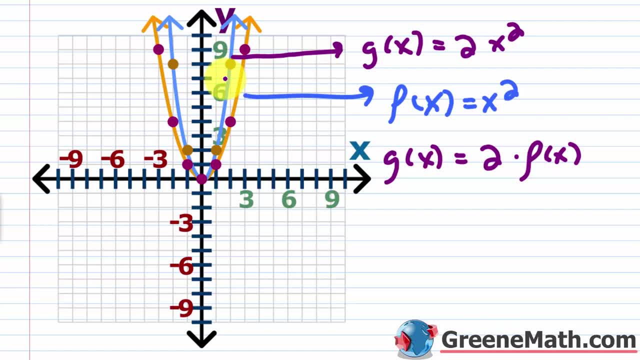 this vertical stretch, OK, this vertical stretch which just means that we are pulling the graph away from the x-axis. A lot of times we like to think about it by saying, OK, well, this point here, originally on, f of x equals x, squared was 2 comma 4.. So let's kind of highlight. 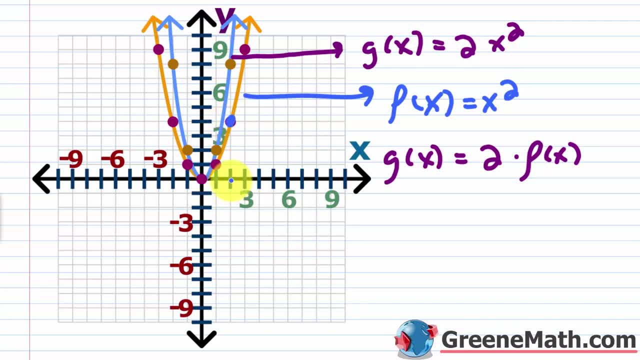 that real quick. Now that same x value of 2 is associated with a y value that is twice as high. So it's up here. So you see how that's pulling the graph away from the x-axis. OK, So that's. 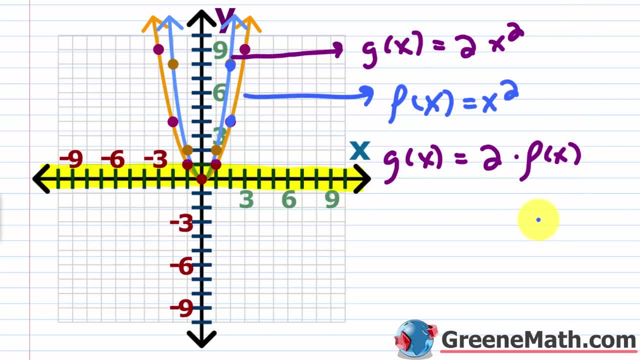 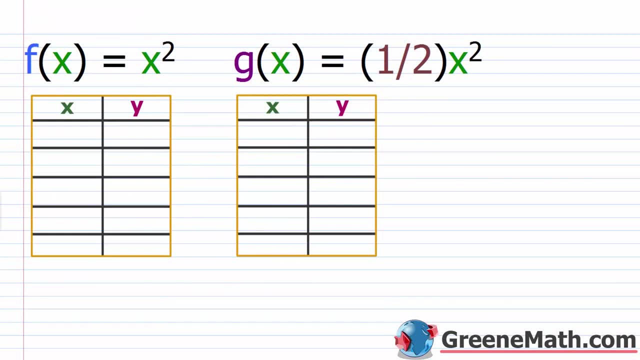 what we talk about when we say that we have a vertical stretch. Again it's being pulled away from the x-axis or the horizontal axis. Now let's look at the other scenario. So we have f of x equals x squared, And now we have g of x is set equal to 1 half times x squared. 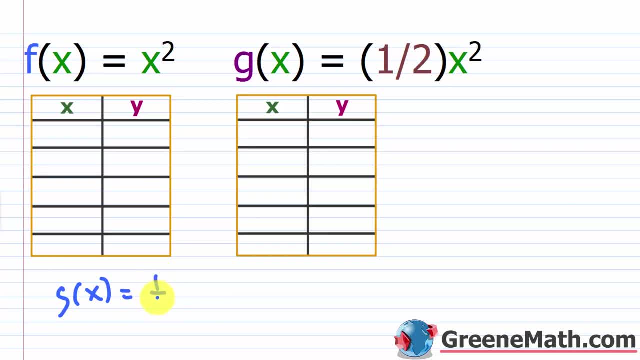 So now what I have is g of x is really 1 half times f of x. Again, f of x is x squared. So 1 half times x squared is this g of x. So what's going to happen is, for a given x value, now my 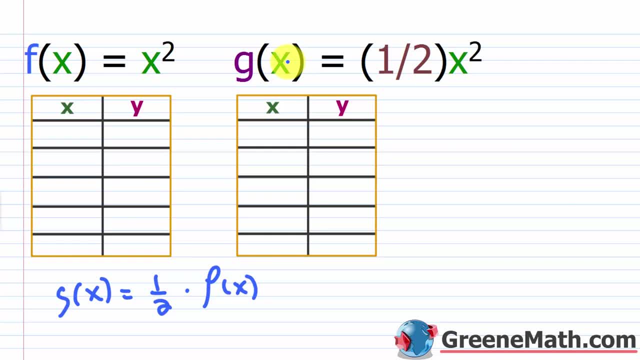 y value is going to be half as large. So instead of having a vertical stretch right where it's narrower or skinnier, right it's being pulled away from the x-axis. Now what we're going to have is we're going to have a vertical shrink or a vertical compression. 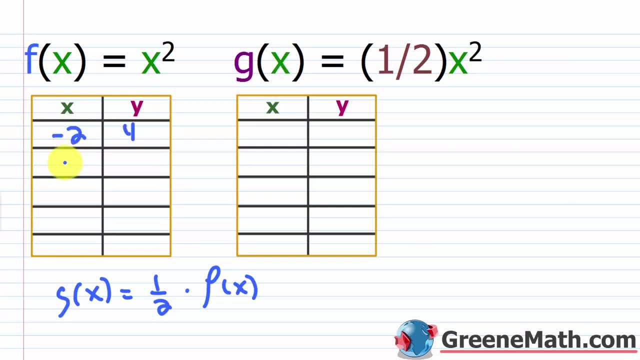 OK. So if this guy again is negative 2, 4,, negative 1, 1,, if it's 0, 0, 1, 1, and 2, 4, these guys, if I stay with the same x values, so negative 2, negative 1, 0, 1, and 2,. 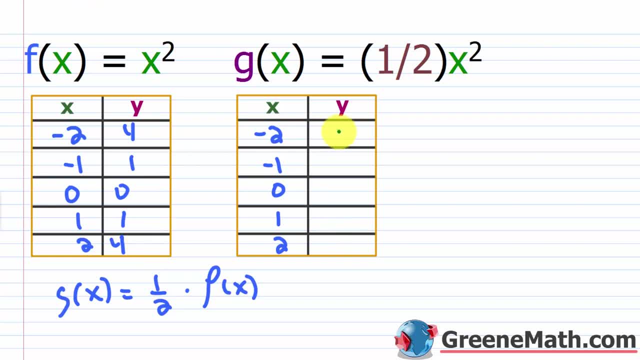 these guys are going to be half as large as these guys, So I would have 2 instead of 4.. I would have 1 half instead of 1.. 0 would be the same right, because 0 times a half is still 0. And then 1,. 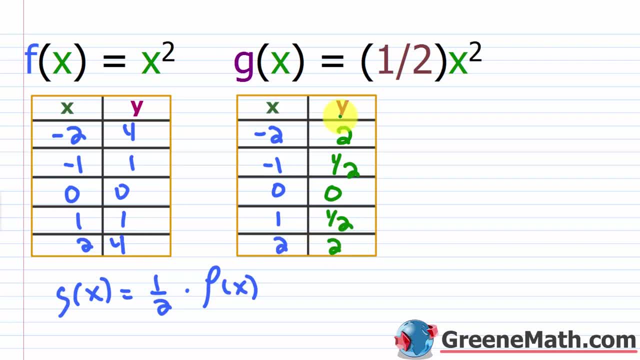 0 would be 1 half, And then 4, that would be 2, right, Everything I did here was I just took these y values and I just multiplied them by a half to get these y values. OK, That's all I did. 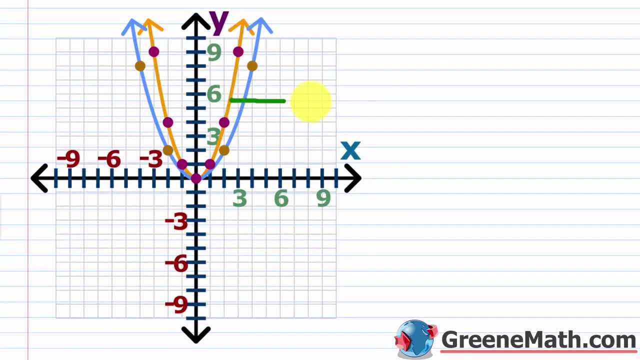 Now, if we look at this visually, we can see that this guy right here is my f of x equals x squared. And then this blue guy: this is my g of x equals 1 half times x squared. OK, 1 half times x squared. 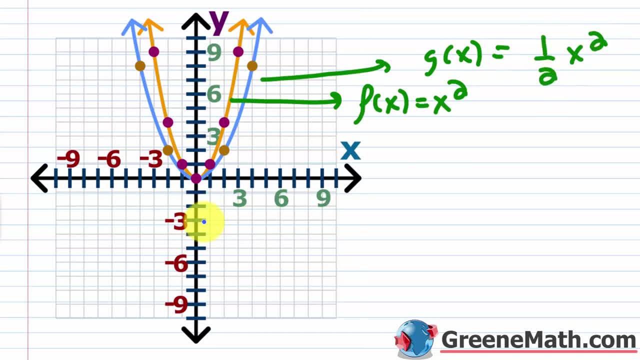 Let me make that a little bit clearer And again let me show you this with a point. So if we have 2, comma 4, that's here Now, the x value of 2 is associated with a y value. that's only 2.. 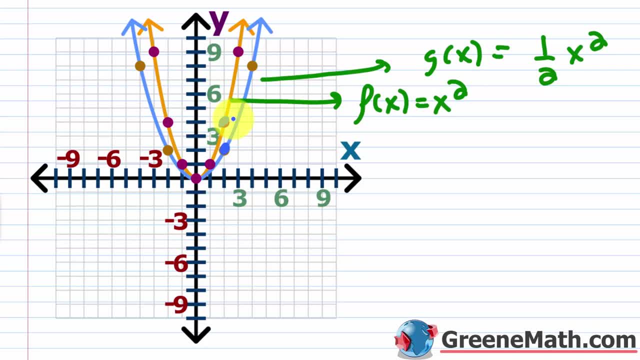 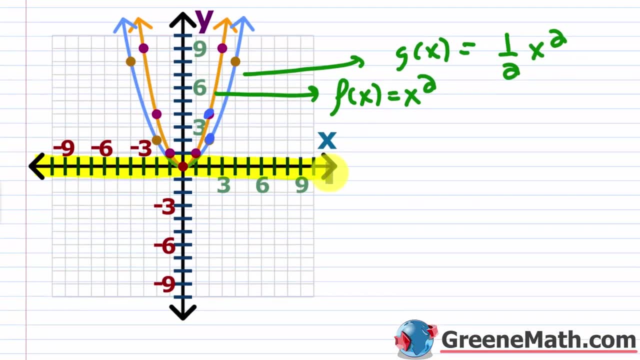 So what happens is this creates a vertical shrink or vertical compression. It's a movement towards the x-axis. OK, It's a movement towards the x-axis, All right. so let's talk about the general rule. This is something you want to write down in your notes And then from here, it's very. 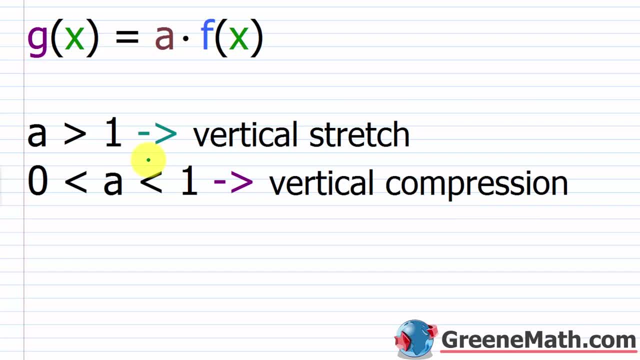 very easy to kind of answer questions about whether there'll be a vertical stretch or vertical shrink, And then also it's easy to kind of graph things. You already know what the parent function looks like. So g of x equals a. OK, some number a times. 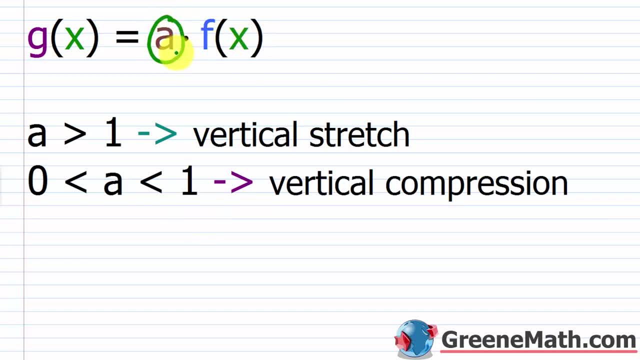 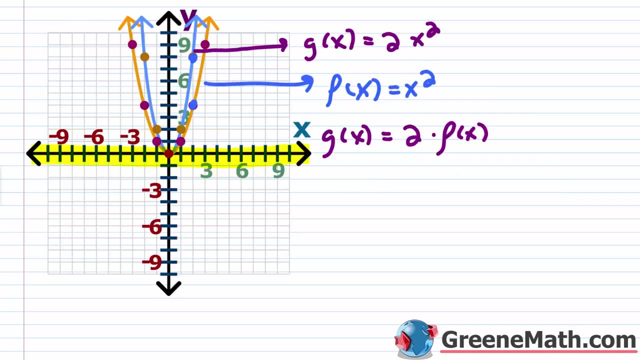 f of x. Now, for the purposes of what we're going to do today, a is going to be positive. OK, I'll talk about negative scenarios when we get to reflection in the next lesson. So a, if it's greater than 1, it's a vertical stretch. We saw that if we had 2 times f of x in this graph here. 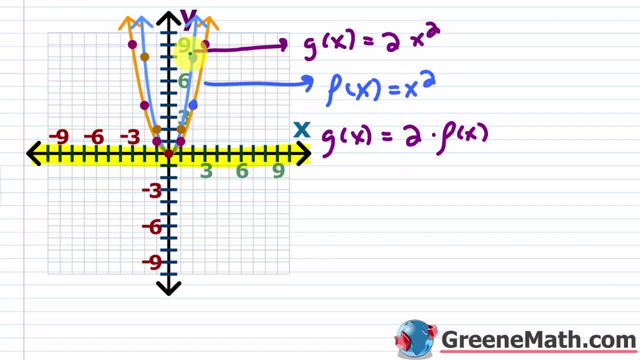 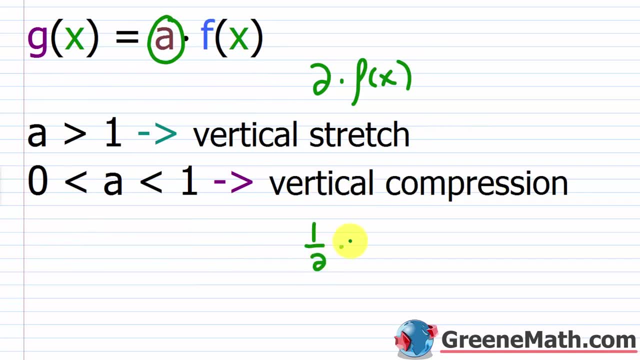 we had a vertical stretch. Again, it was a movement away from the x-axis. Then, if a is greater than 0 and less than 1, we're going to have a vertical compression right. We saw this with 1 half times f of x. We can see that here, Again, we had a movement towards. 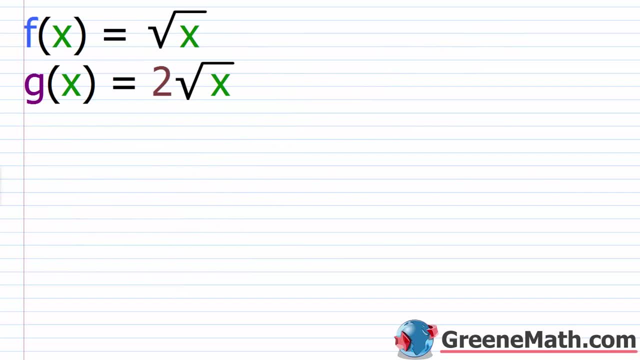 the x-axis. All right, so suppose we look at: f of x equals the square root of x, and then g of x is equal to 2 times the square root of x. So really, again, g of x can be defined as 2 times f of x. 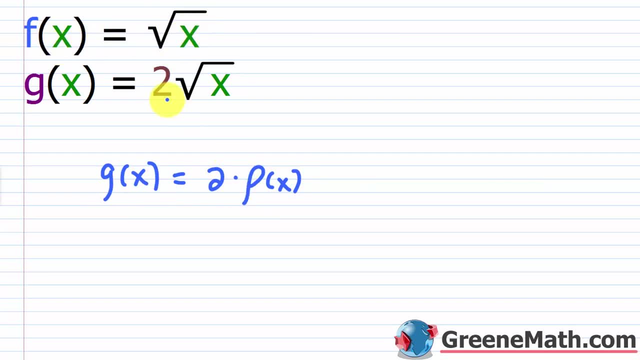 OK, That's all it is, because f of x is the square root of x. Well, 2 times the square root of x, 2 times f of x, right, That's what g of x is. So what's going to happen is for a given x value, 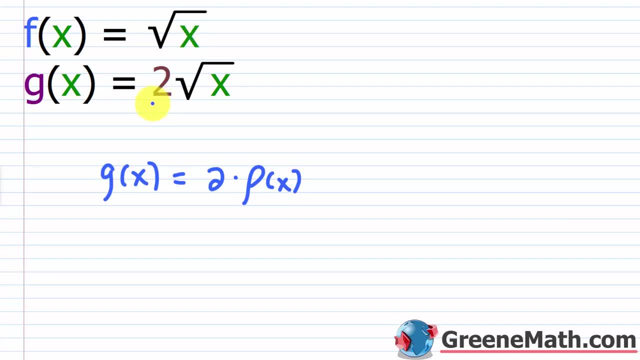 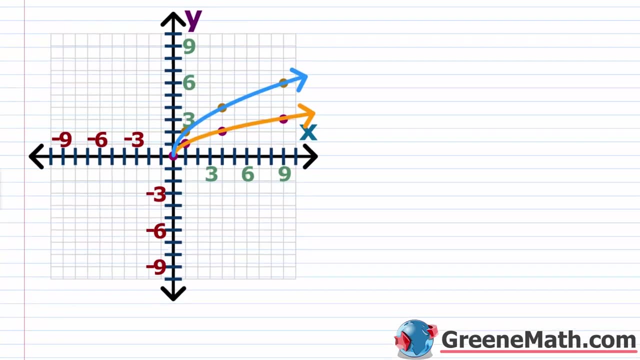 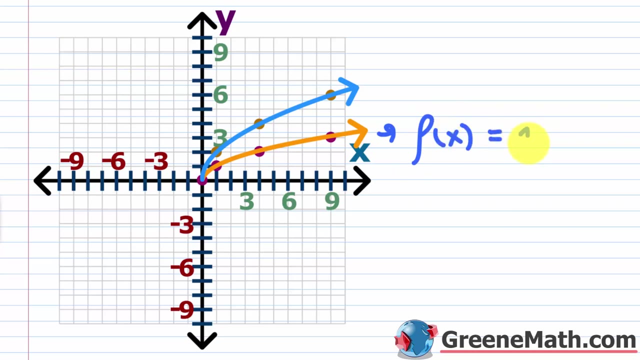 the y value is now twice as large right, I can just multiply it by 2. So this will give me a vertical stretch right, or a movement away from the x-axis. So if we look at the two graphs here, this guy is the graph of f, of x is equal to the square root of x. Then this guy here is going to: 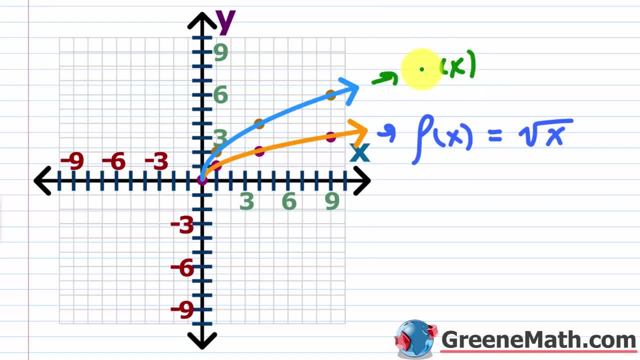 be g of x. Let me make that g a little bit better. The g of x is equal to the square root of x, is equal to, again, 2 times the square root of x. So the way to graph this kind of quickly. 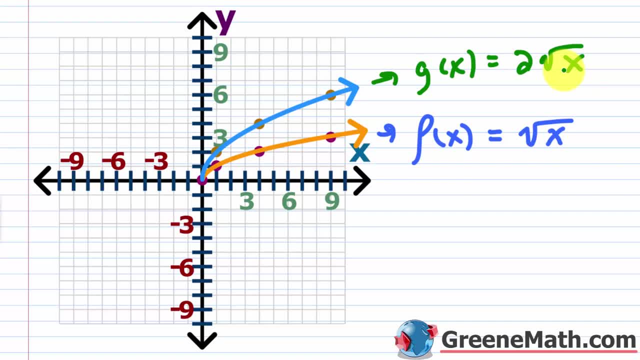 if you don't want to use kind of like a t-table or something like that. if you already know f of x equals square root of x, if you already know what that looks like, then essentially what happens is you take each y value, OK. for the same x value, you just multiply it by 2.. So 0 comma 0 is still. 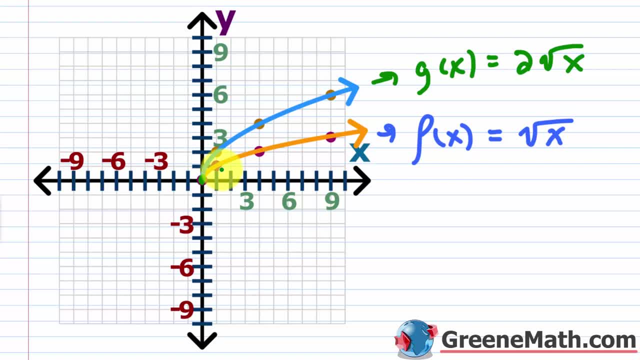 there, OK. But if I go to 1,, right, I know that square root of 1 is 1.. So that's this point here: 1 comma 1.. But now in the g of x function, if I take the square root of 1, I get 1, but now I multiply it by 2.. So now I have an x value of 1. 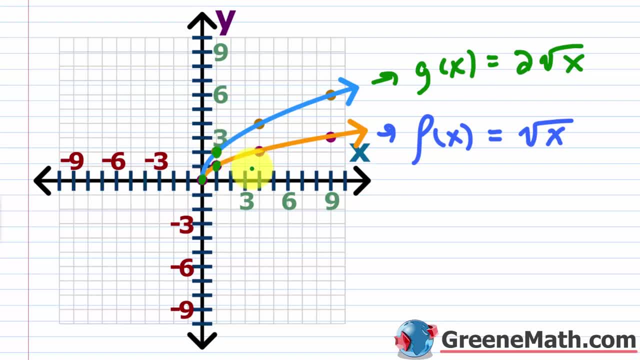 corresponding to a y value of 2.. And as we move to the right, this point here, that's 4 comma 2, would now be 4 comma 4, right, Because I took that y value of 2 and multiplied it by 2 to get a y. 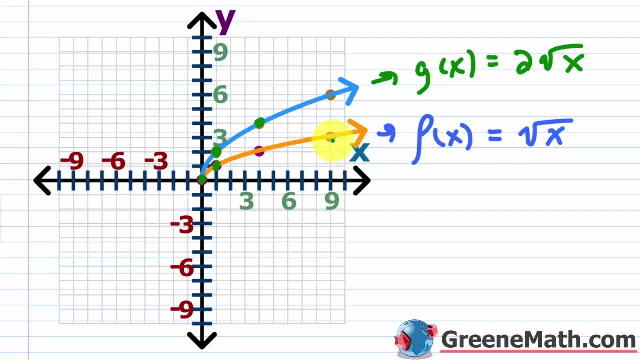 value of 4.. And here, where we have 9 comma 3, just multiply the y value of 3 by 2 to get 6.. So now it would be 9 comma 6.. So once you have these kind of four points, you can sketch the. 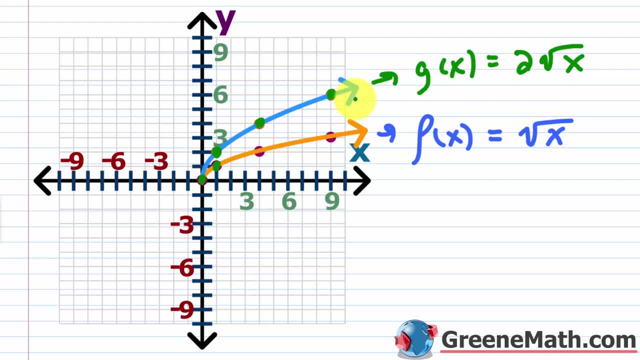 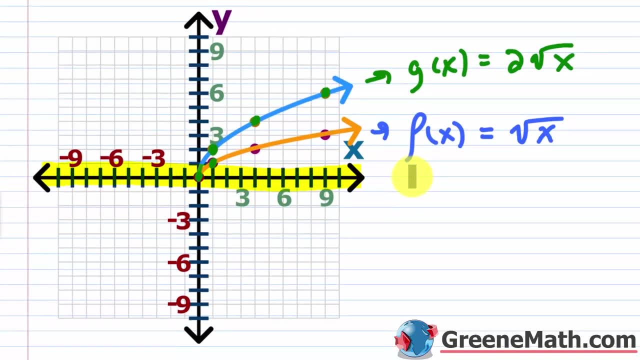 g of x very, very quickly, right. But the main thing here is to understand that you have a vertical stretch here or again a movement away- OK, a movement away from the x-axis, All right. so now let's look at: f of x equals the absolute value of x, and then g of x equals: 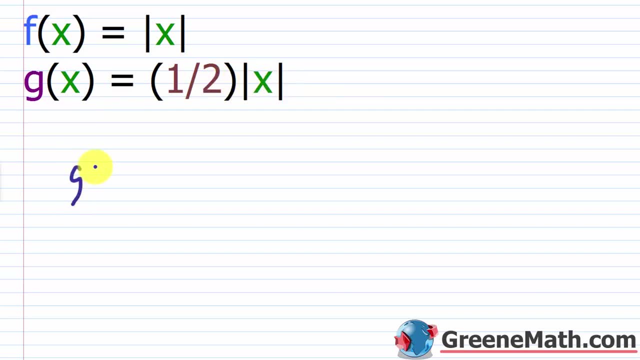 1 half times the absolute value of x. So again, g of x can be defined as what I've got. this 1 half, that is multiplying f of x. right, f of x is the absolute value of x. 1 half is multiplying f of x. 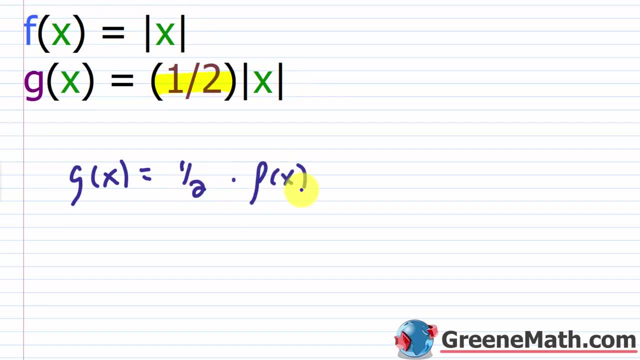 So g of x is 1 half times the absolute value of x. So g of x is 1 half times the absolute value of x. So we know at this point, because this guy is between 0 and 1, it's going to create a vertical. 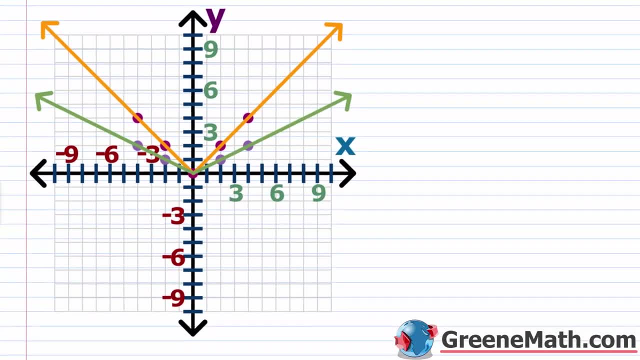 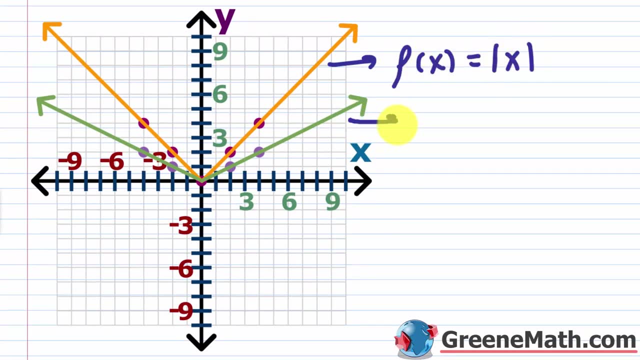 compression or a vertical shrink. So looking at this guy, this is the original f of x equals absolute value of x. Then this guy right here is what It's: g of x is equal to 1 half times the absolute value of x. So again, thinking about this, if I want to graph it quickly without a t, 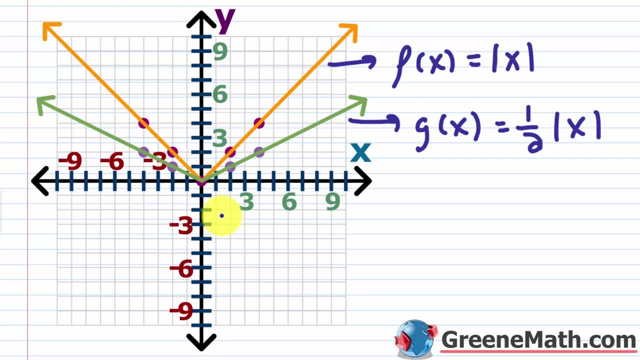 table for a given x value, the y value is now 1 half times the absolute value of x. So again thinking about this, if I want to graph it quickly without a t table, for a given x value, the y value is now 1 half. 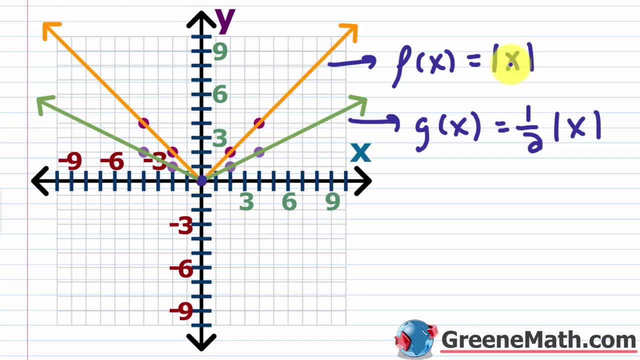 So g of x is 1 half times the absolute value of x. So g of x is 1 half times the absolute value of x. So 0 and 0 is still going to be there, right? Because if I plug in a 0, I get 0.. 0 times a half is still 0. 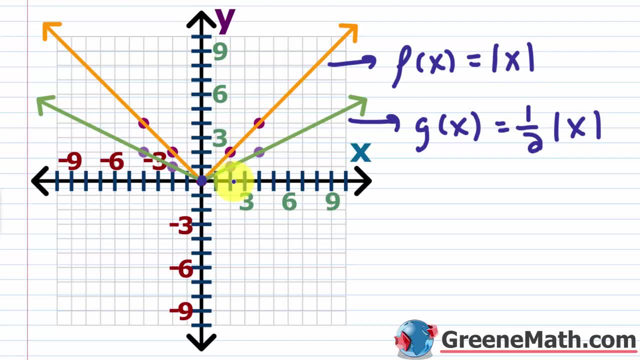 But if I move out, let's say I do 2.. Well, 2 is associated with a y value of 2 here, okay, But in the new g of x I just cut it in half, And so 2 is associated with a y value of 1.. 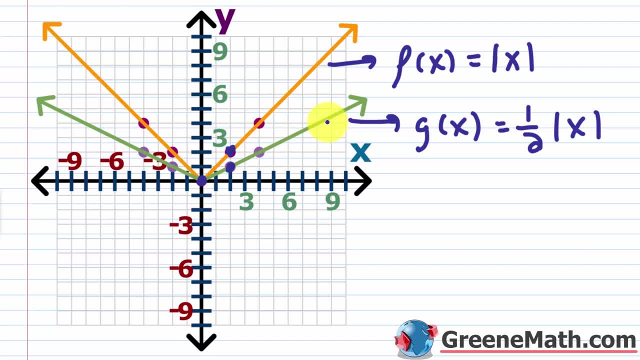 You can just keep doing this to get enough points to kind of graph this pretty quickly. But one of the main things is to understand that you would have a vertical compression here, because this number right here, that's multiplying f of x, is going to be between zero and one. right It's greater. 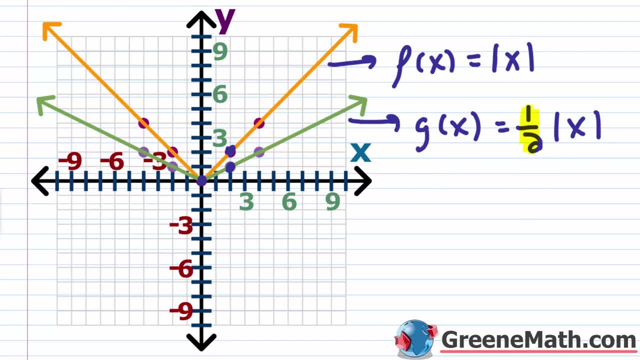 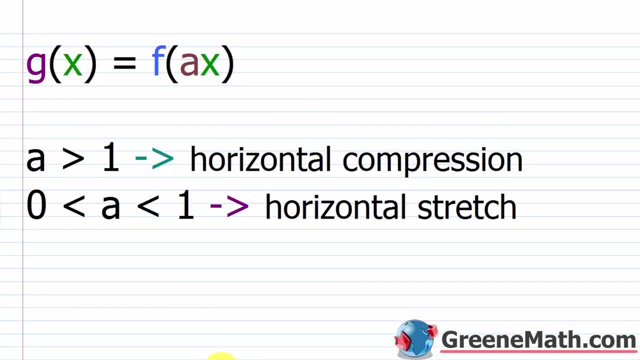 than zero and less than one. So that's what's creating this kind of vertical compression or movement towards the x-axis. All right, so we're also going to come across horizontal stretching and compression. So, with a horizontal stretch, now it's going to be a stretching of the graph. 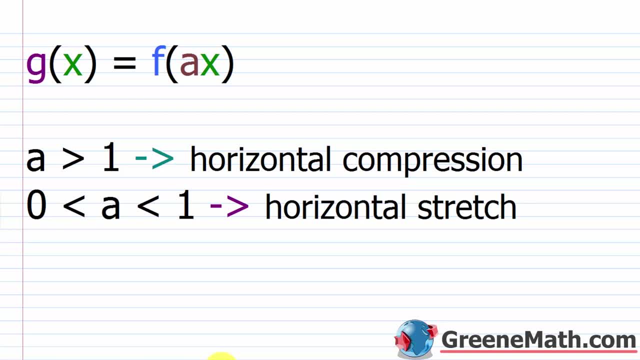 away from the y-axis. okay, We saw, with a vertical stretch, we stretched the graph away from the x-axis With a horizontal stretch, we're now stretching it away from the y-axis. okay, With a horizontal compression, this is now going to be a squeezing or compression of the graph towards the y-axis. 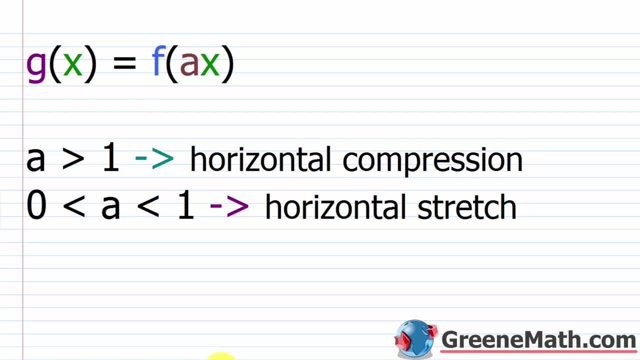 Again, with a vertical compression, we were compressing it towards the x-axis. Now, with a horizontal compression, we are compressing it towards the y-axis. Now what's going to happen is we have g of x that's defined as being equal to f of ax. So let's think about this notation. 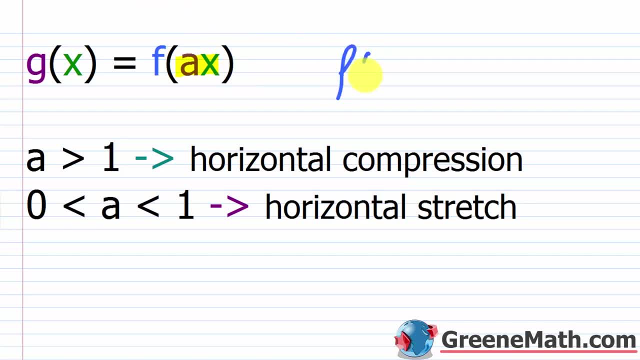 for a minute. So let's think about this notation for a minute. So let's think about this notation for a minute. I know we've all seen this at this point, If we see something like f of 2, we know we just plug in a 2 for each occurrence of x and f of x, So this is no more challenging. 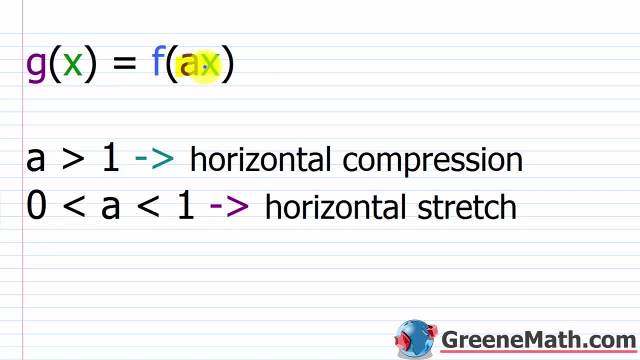 I just take ax, plug it in for each occurrence of x and f of x. So if I had something like, let's say, f of 2x, let's say I had that Wherever I have an x in my function, just plug in a 2x, That's all. 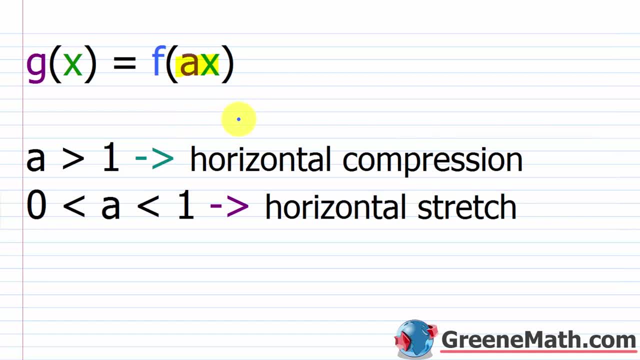 it is okay, Nothing fancy. Now here comes the confusing part, and I'm just going to tell you in advance: it's a little bit more challenging to understand a horizontal stretch and a horizontal compression versus a vertical stretch and a vertical compression. What's going to happen is: 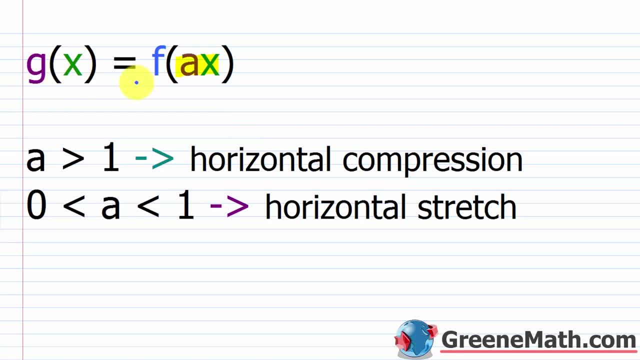 to obtain this g of x based on our original function f of x, we can essentially just multiply each x coordinate of that original function by 1 over a. So let me write that down: So 1 over a. And this part's going to be confusing. We'll see when we get to the example that it takes a minute. 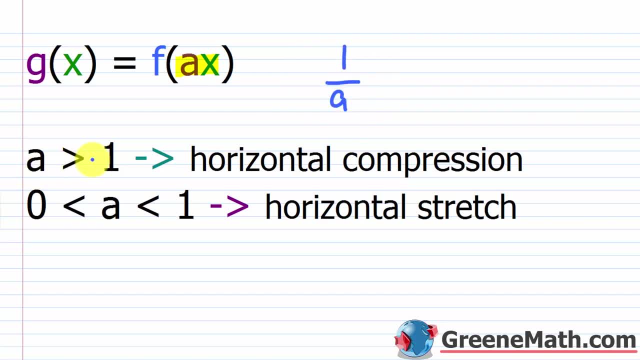 to kind of wrap your head around where this comes from. So if a is greater than 1, now we're going to have a horizontal compression, And if a is greater than 0, we're going to have a horizontal stretch. So the first thing that makes it confusing, it's kind of hard to keep track of. 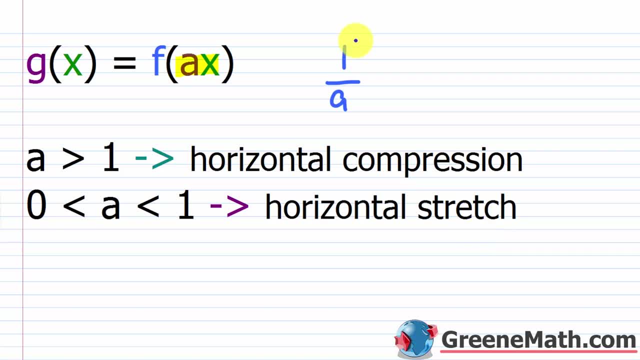 kind of what's going on. okay. And the second thing is this: 1 over a is really confusing. Where did this come from and why does this kind of happen? Essentially for a given y value. now the x values are obtained by kind of taking those x values from f of x and multiplying them by this. 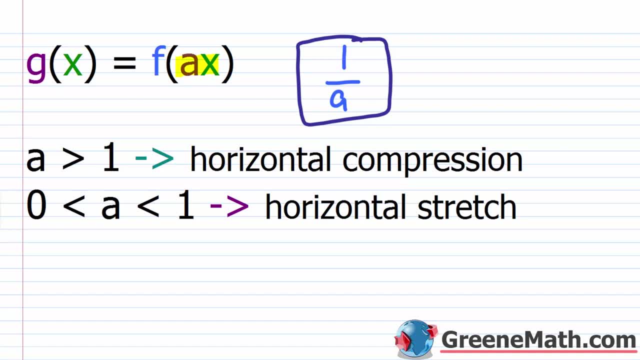 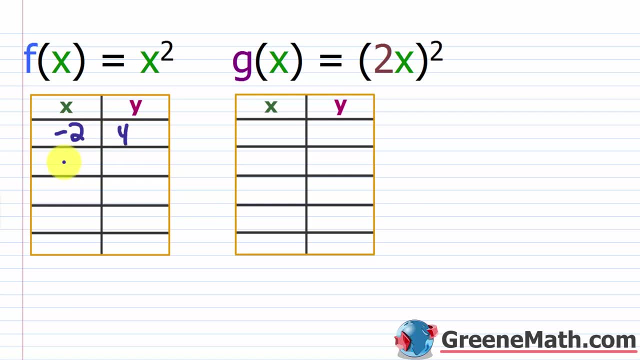 1 over a. So let's look at an example so this can be more clear. So we have f of x equals x squared. We've committed the points to memory. So we know negative 2, 4.. We know negative 1, 1, 0, 0, 1, 1,. 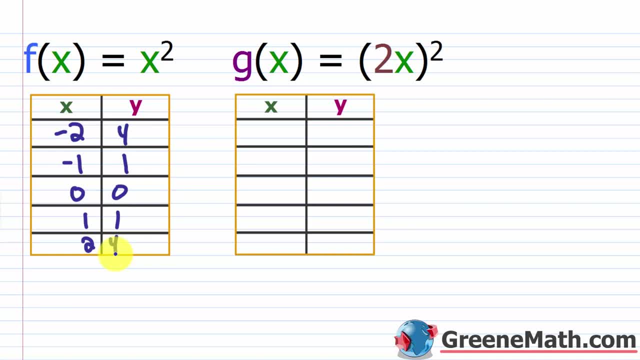 and 2, 4.. But essentially, what I just told you was that for this g of x, here it's equal to this 2x, and this is being squared. Well, what I can write, this, as is what This guy right here is essentially. 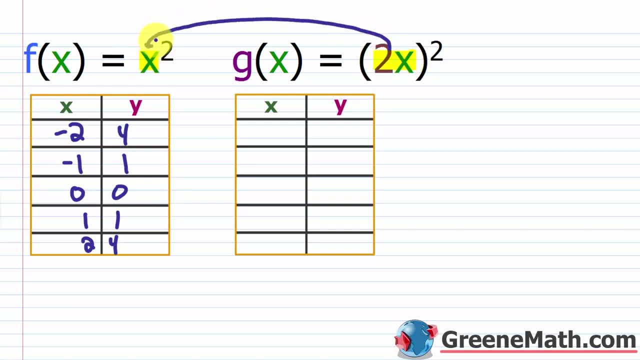 just plugged in for x. This guy is plugged in for x. So what I can say is that I have g of x being defined as f of this 2x, Okay, this 2x, And notice that it's this 2 that's multiplying the x. So this is my value. 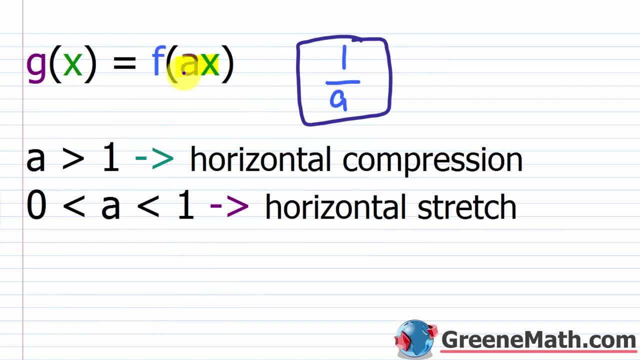 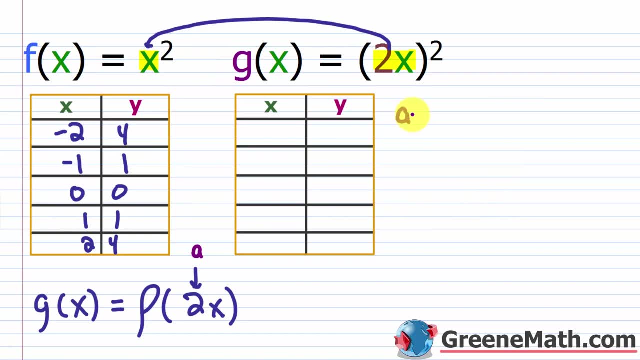 for a. Okay, that's my value for a. If I go back, it's a times x, that's inside these kind of parentheses. In this case, that value is going to be 2.. Okay, so let me write this off to the. 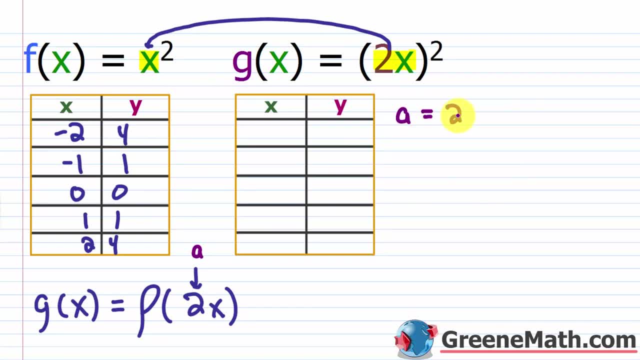 side. Just say a is 2.. Now I told you that for a given y value I can find kind of the new x values that's associated with this g of x by taking these x values and multiplying them by 1 over a. 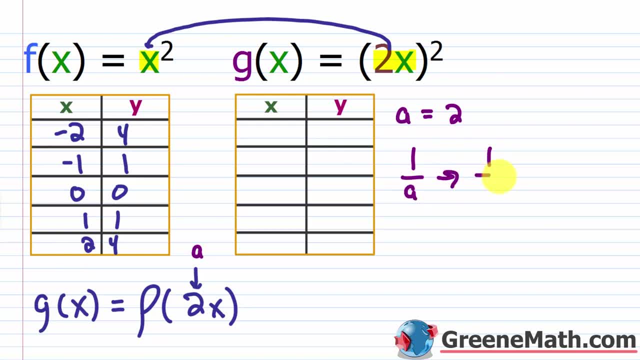 In this case, a is 2.. So 1 over a is going to be 1 over 2 or 1 half, And this is the part that's going to be tricky. It's not going to make sense at first, So let's copy these y values We have. 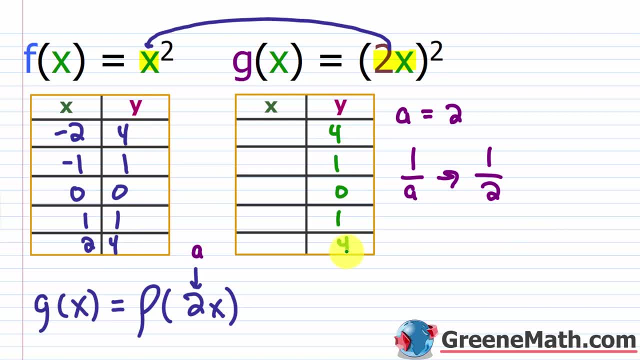 4,, 1,, 0,, 1, and 4.. And then I'm going to just find my x values by kind of taking these and multiplying them by a half. So let's put times 1: half there. That kind of looks like an x, So let 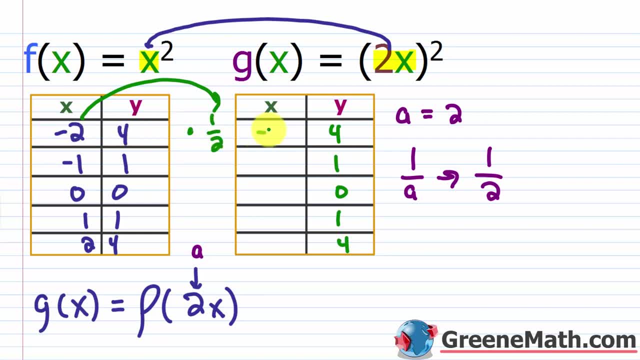 me just put a times like that. So negative 2 times a half is going to be negative 1.. Negative 1 times a half is going to be negative. 1 half. 0 times a half is still 0.. 1 times a half is 1 half, And then 2 times a half is 1.. Okay, so the 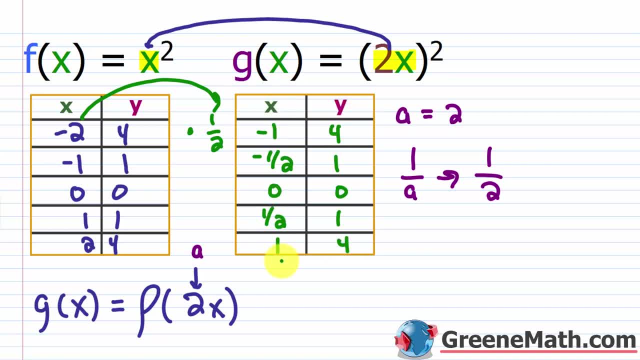 intuition here is that for a given y value, the x value should have been doubled. right, Because this guy is a 2.. But in fact they were cut in half. So what caused that? Well, what's going on here is that- let me kind of erase this for a second- We have this 2 here that is multiplying x. 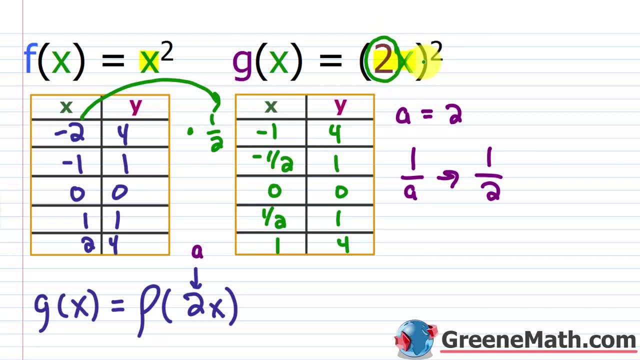 before it gets squared. okay, So now what's going to happen is this: y value is associated with an x value that is half as large as it was before. Again, this is really tricky to wrap your head around at first, But if you think about it, the 1 half. 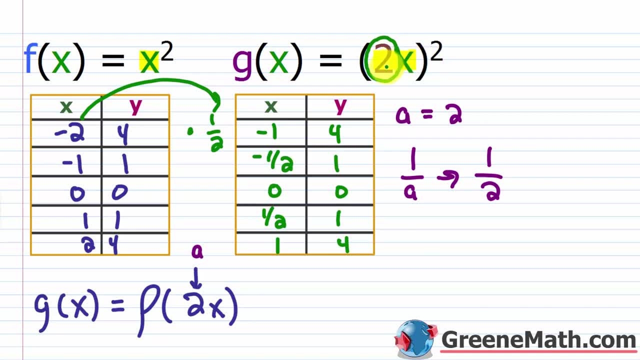 is just what's needed to kind of undo this multiplication by 2 and get this kind of new x value that's associated with that y value. So in this example, if x is 1, y is 1.. But here, if y is 1,, well, x needs to be 1 half, And the reason for that is I have 1 half. that gets. 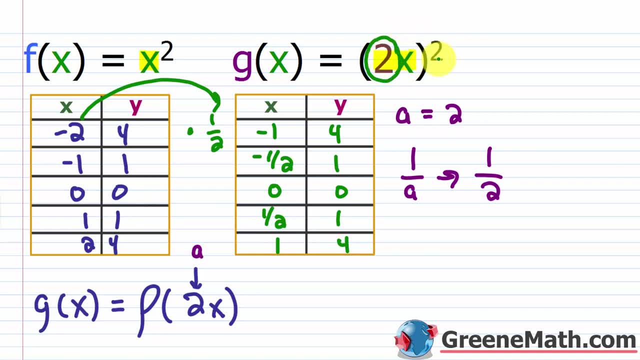 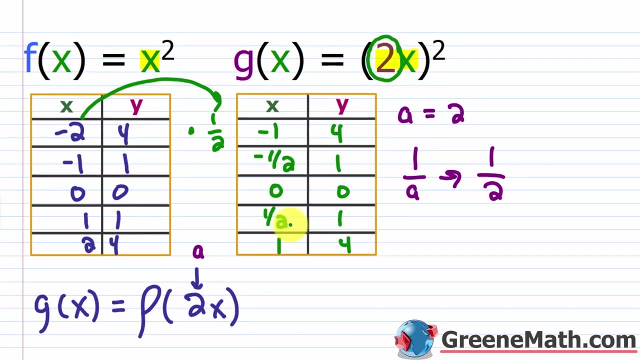 multiplied by 2 first, And then it's squared. So what's going to happen is, because of this, we have that same y value that's associated with an x value that's half as large. This is compressing the graph horizontally, or moving it towards the y axis. So let's look at the graphs. So this is going to be my original. 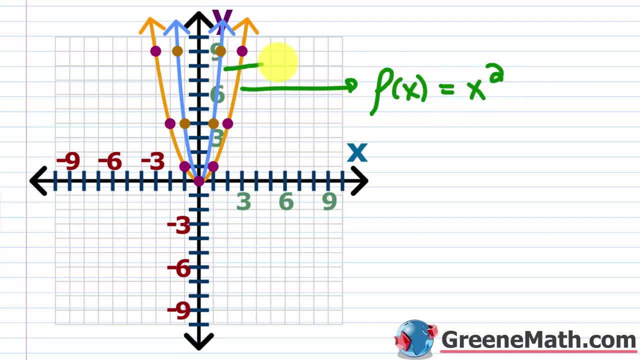 f of x equals x squared. And then in blue we have our g of x, which is equal to 2x, And this amount is squared. So let's just take a point right. Let's just take, let's say this, 2 comma 4.. So this 2 comma 4 on the original f of x equals x squared. 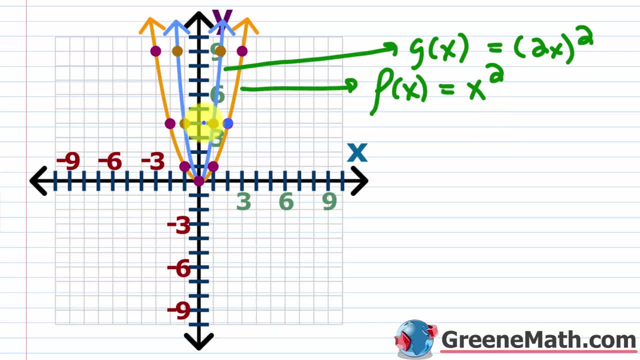 Well, now what's going to happen is this: y value of 4 is associated with an x value of 1 now instead of 2.. And I know it's also associated over here on the left, but let's just focus with these points right here on the right. So what's happening is we're getting a horizontal compression. 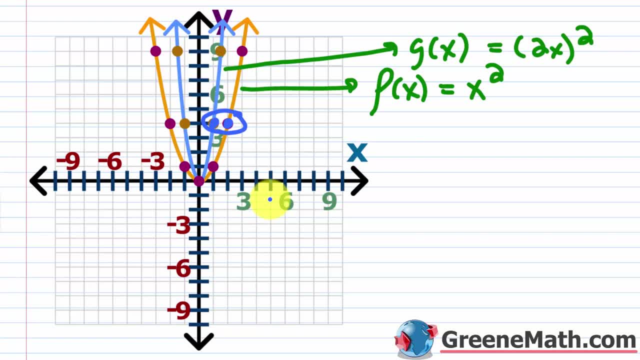 or a movement towards this y axis, Because again we have this 2 that is multiplied by 2. And so we're applying x before it gets squared, okay, So that y value is now associated with an x value that is half as large. okay, So that's what's going on there. Now let me kind of address a point of 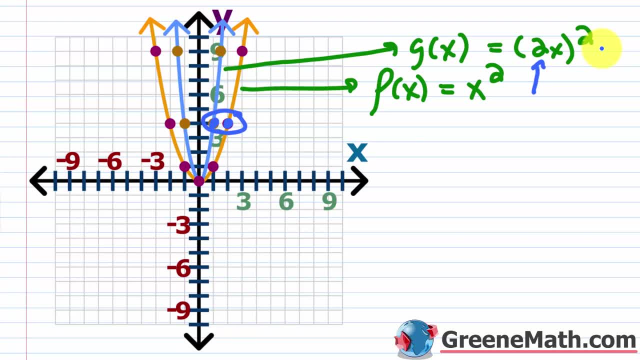 some confusion. You might be scratching your head and telling me that this graph is stretched vertically. Well, in fact, you would be correct, because in this particular case it does work out, because we could say that, really, g of x is what. If I squared 2, I would have 4.. If I squared x, 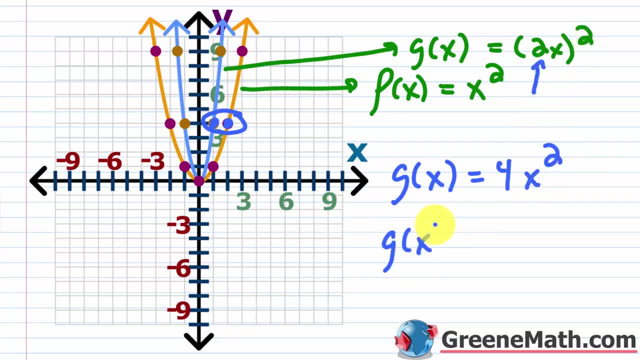 I'd have x squared. Well, I can also say that g of x is really just 4 times f of x, right, If f of x is x squared. So if I look at- let me kind of erase this- If I look at this this way, well, really, for a given. 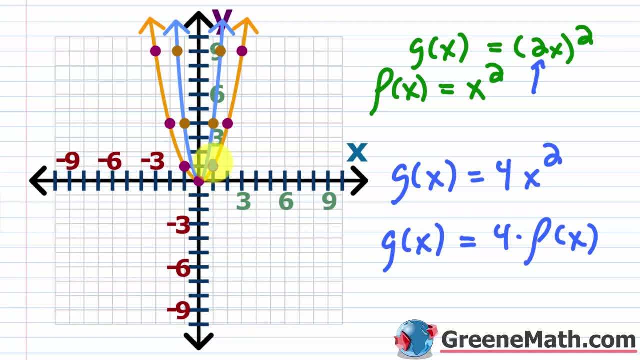 point. let's say I chose the point 1 comma 1 on the original. Well, now that x value is associated with a y value that's 4 times as large, right, 1 comma 4.. But I want you to kind of not get into. 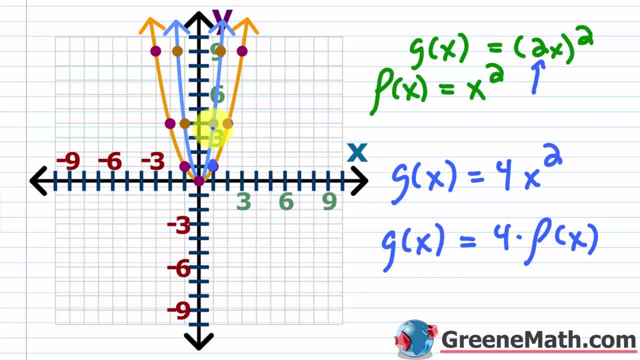 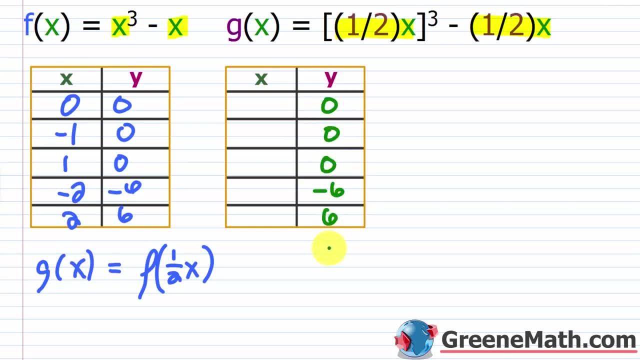 again negative six and six for these, given y values, I can just take the x values that are associated and I can just multiply them by one over a, In this case my a- the guy that's multiplying the x- is one half. So one over one half is what this is. division with fractions. 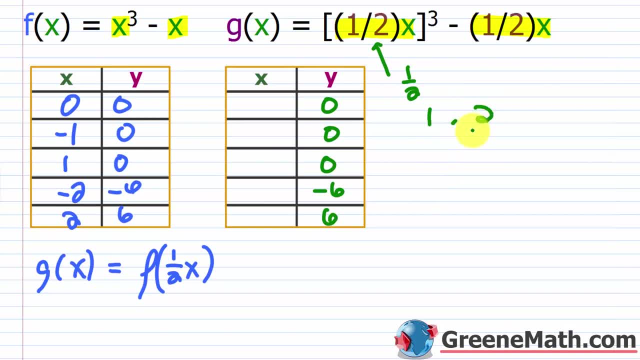 it's basically one times two over one, which is just two. Okay, so now what's going to happen is I'm going to multiply each of these guys by two. So zero times two is still zero negative. one times two is negative two. one times two is two negative. two times two is negative. four and two times two. 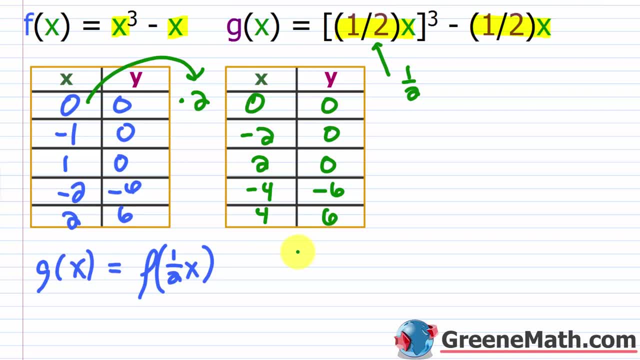 is four. So we have all these points here that are going to be associated with this kind of g of x function. And again, for a given y value, the x values have just been multiplied by two from that f of x function. So what's going to happen is we are going to horizontally stretch. 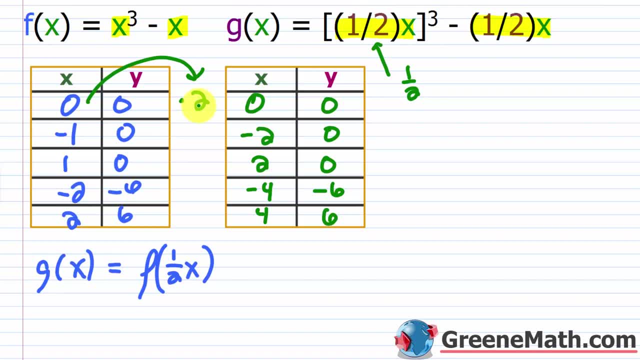 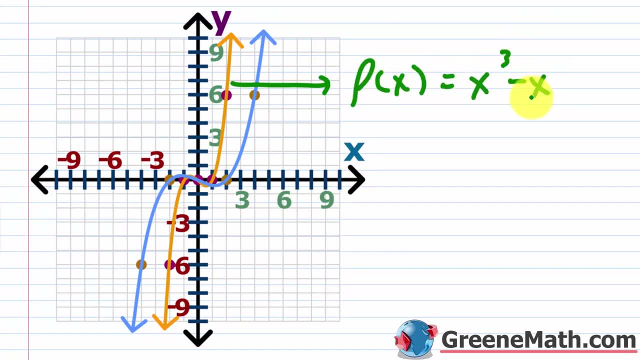 the x values. So what's going to happen is we are going to horizontally stretch the x values. Okay, we're going to horizontally stretch this function. So let's take a look. So we've already kind of plotted the points and sketched everything. This guy is: f of x equals x cubed minus x. 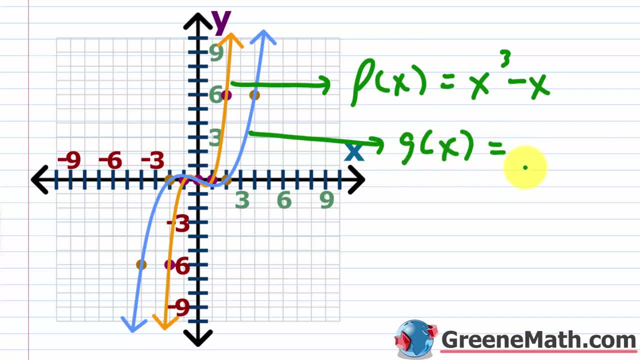 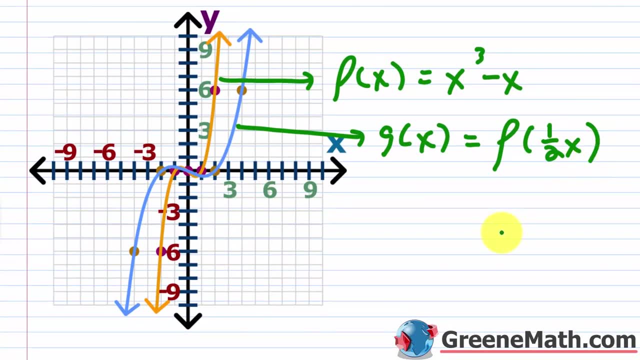 And this guy in blue is g of x is equal to. let's just go ahead and say it's f of one half x, to make it a little bit more simple. And essentially what I see is that what. let's say: I take an x. 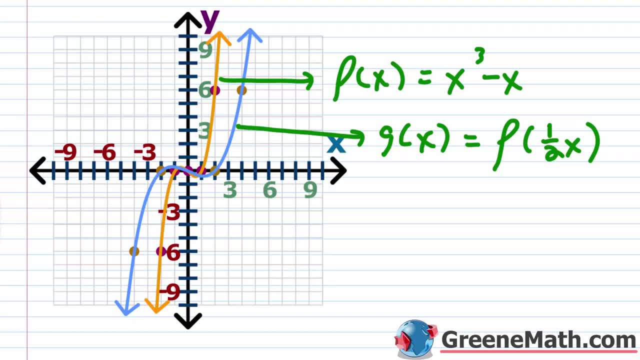 value of positive two. Well, here it's associated with a y value of six. Well, now, that same y value of six is associated with an x value that's twice as large, right? So this guy over here, this x value is four. So you can see that this guy has. 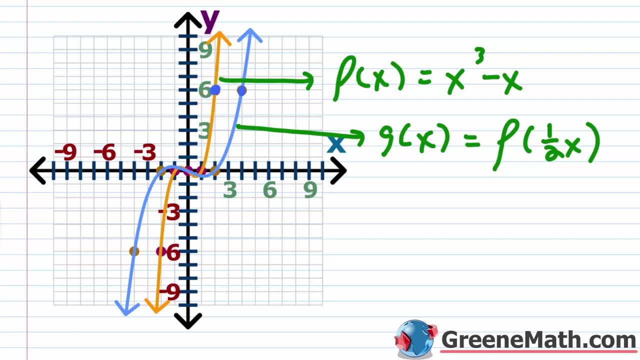 been horizontally stretched right. It's moving away from the y axis. So that's what's going on, And it's by a factor of again one over this, one over one half, which is two. So when you work with this horizontal stretch and horizontal compression, you've got to be able to keep this straight in. 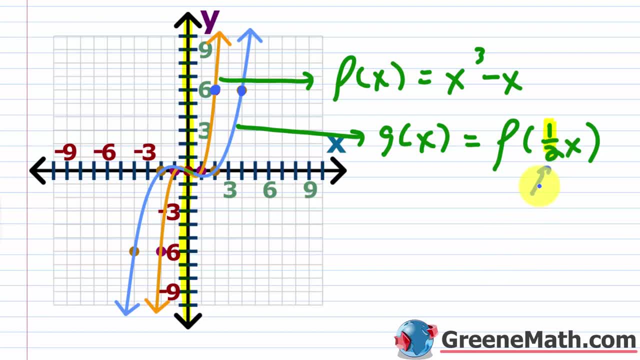 your mind. You've got to remember that this guy right here, this ends up being a okay, And it stretches it horizontally by a factor of one over a. So what happens is, if a is going to be kind of larger than one, then you're going to end up with a fraction here, right, You're going to end up with